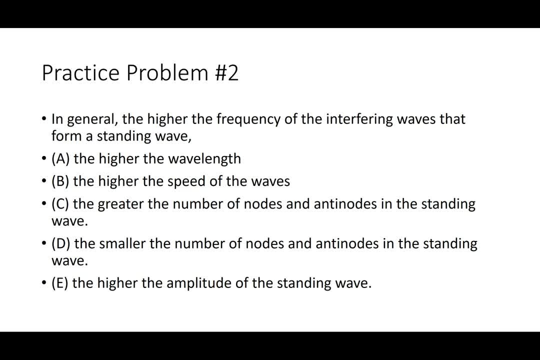 interfering waves that form a standing wave go blank. First of all, the higher frequency doesn't necessarily have anything to do with a higher wavelength, not necessarily a higher speed, Because the wavelength could get shorter. what it does have to do with is C, if the 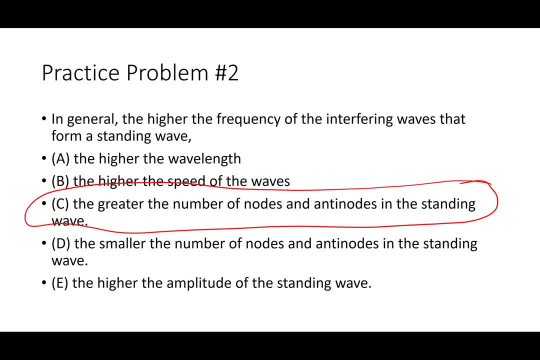 frequency is higher, that means there's going to be the interference between the two waves is going to occur more often and that means there's going to be more points of complete destructive interference, which are nodes, and more points of complete constructive interference, which are antinodes. so C is 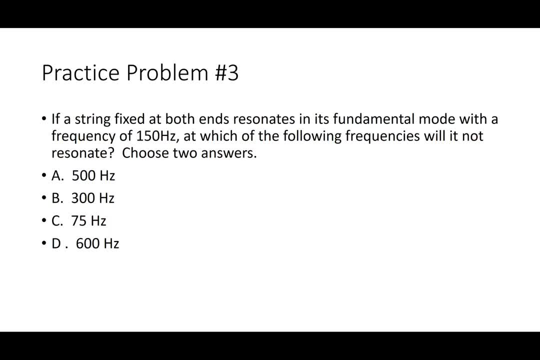 our correct answer on practice problem number two. all right, here's practice problem number three. if a string fixed at both ends resonates in its fundamental mode- and remember that fundamental mode is the lowest frequency- it's the first harmonic that it will vibrate at. that frequency is 150 Hertz. 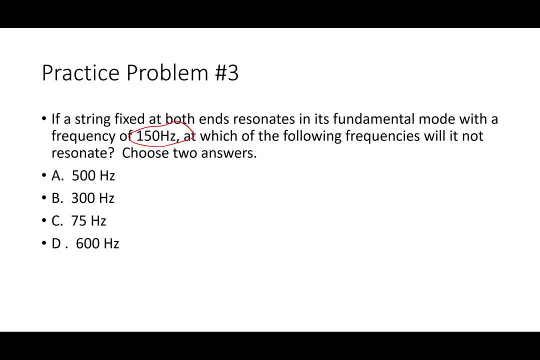 at which of the following frequencies will it not resonate? first of all, it won't resonate it at a frequency lower than the fundamental, so that means 75. it will not resonate at 75 because those are multiples of 150. it will not resonate at 500 because 500 is. 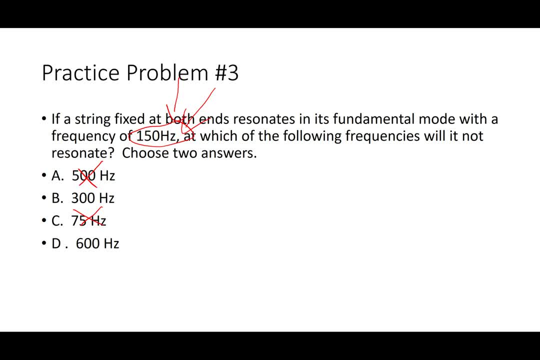 not a whole number multiple of 150.. So the question here asks us which of the following frequencies will it not resonate at, and those are A and C. C because the frequency is lower than the fundamental frequency, and A because 500 is not a whole number multiple of that fundamental 150. All. 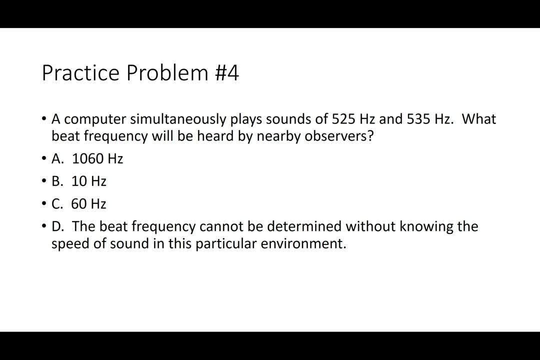 right. here's practice problem number four: A computer simultaneously plays sounds of 525 Hertz and 535 Hertz. What beat frequency will be heard by nearby observers? So when two sounds that are close in frequency are played simultaneously, there's going to be this pattern of constructive and destructive. 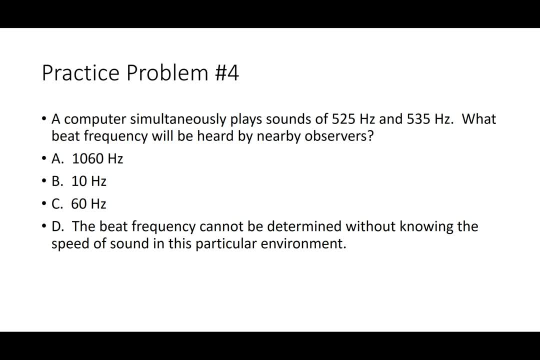 interference. When the waves destructively interfere, the sounds gonna get quieter. When they constructively interfere, the sounds gonna get louder. To determine the actual frequency of the beat that you will hear, you subtract the frequency of the sound And then you subtract the frequency of the sound. So 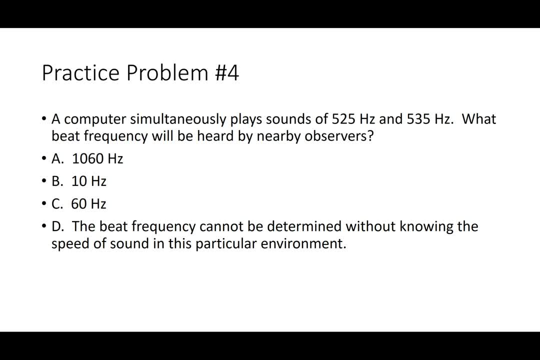 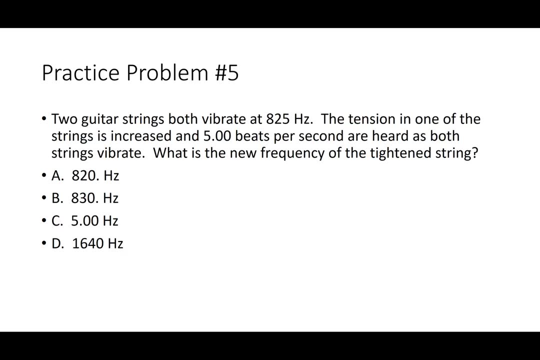 of the two sounds. So in this case we're going to go 535 Hertz minus 525 Hertz and we're going to end up with a beat frequency of 10 Hertz, So we should hear 10 beats per second. Alright, practice problem five: Two guitar strings both. 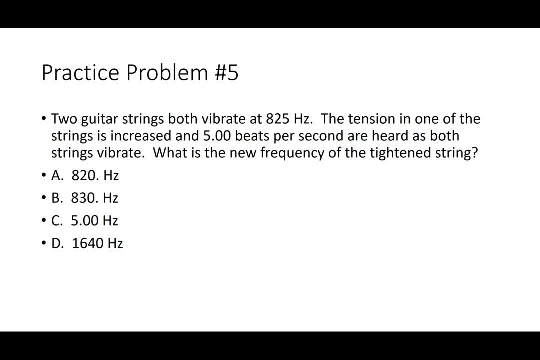 vibrate at 825 Hertz, The tension in one of the strings is increased and five beats per second are heard as both strings vibrate. What is the new frequency of the Titan string? Alright, when a string has more tension in it, that increases the speed of the wave. Well, in this case, because the wave is 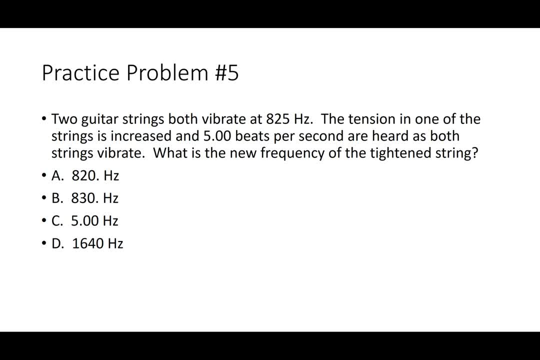 moving faster, it's also going to have a higher frequency. Now we're going to have two waves nearby of simultaneously being played- one in each string- and they're going to start to interfere, and that's how we're going to get the beats. Now we 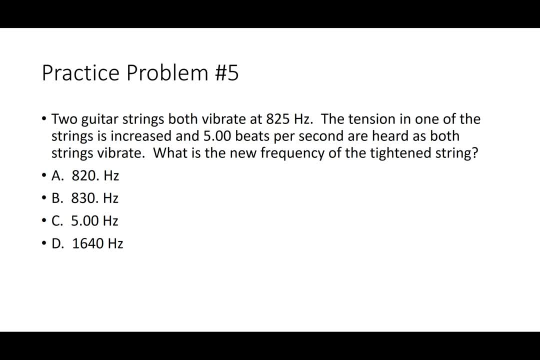 saw in the last problem, to find the beat frequency we're going to subtract the frequencies of the second string. So the third string is the higher frequency of the two sounds. We know in this case the difference in frequency is five. We also know that the that 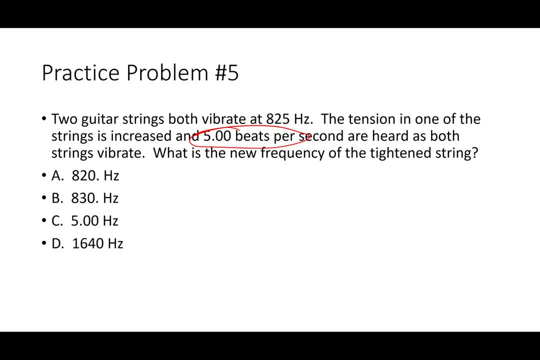 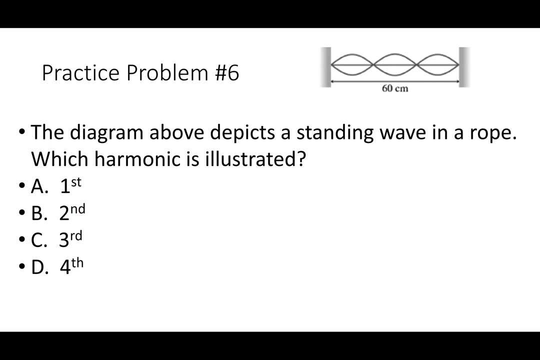 frequency in the Titan string is going to be higher than it was to begin with. It was 825, now it's going to be higher, So the new frequency of the Titan string is going to be 830 hertz. Answer B looks good on practice problem number five. All right, practice problem six: The diagram. 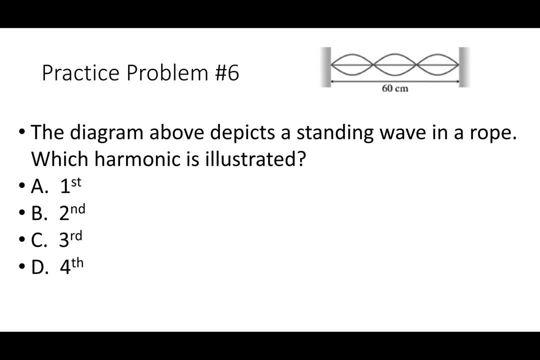 above depicts a standing wave in a rope, which harmonic is illustrated. You can determine the harmonic number by counting the antinodes, the points of maximum constructive interference. So here's an antinode: one, two, three. this is the third harmonic. 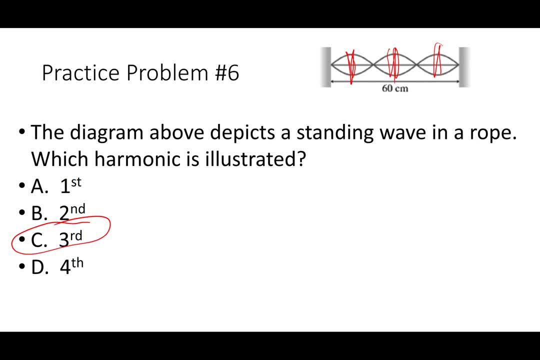 so the number of antinodes is going to be equal to the harmonic number. The number of nodes- in this case the points of destructive interference, one, two, three, four- the number of nodes is always one higher than the harmonic number. All right, so here's another standing. 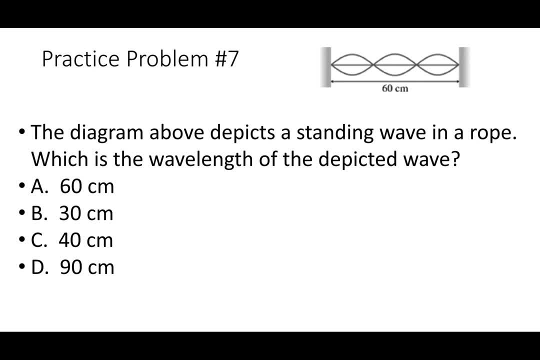 wave problem. The diagram above depicts a standing wave and a rope. What is the wavelength of the depicted wave? Well, remember, one complete wavelength in a standing wave is two of these loops. We know the string length is 60 centimeters, So one of our waves is essentially two-thirds of. 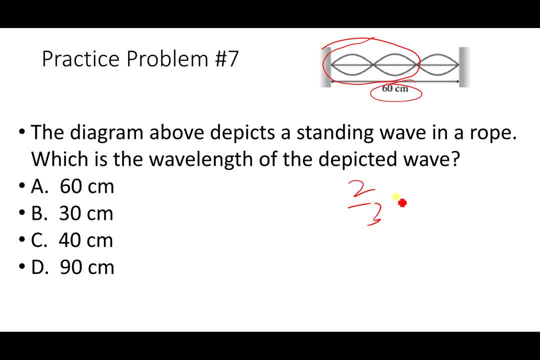 the string length. So we're going to take two-thirds of 60, and two-thirds of 60 is going to end up being 40. We're in centimeters, So our wavelength for this particular wave is 40 centimeters. One wavelength in this case is two-thirds of the string length And again, 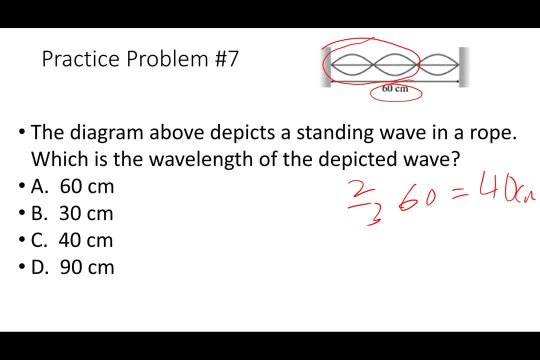 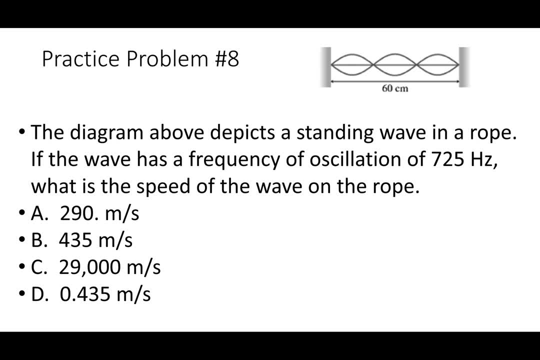 remember that one wavelength is two loops in a standing wave. All right, this problem is related to practice problem seven. Here we have the same standing wave that we had in seven. We know the wave has a frequency of 725 hertz and we want to know the speed of the wave in the 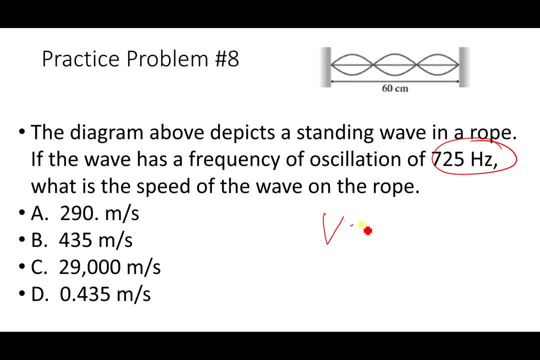 rope Again. this time we're going to have to use the wave equation, which is: speed is equal to wavelength times frequency. In the previous problem we found that the wavelength two loops is equal to two-thirds of the string length, 60. So that was 40 centimeters. So our wavelength is. 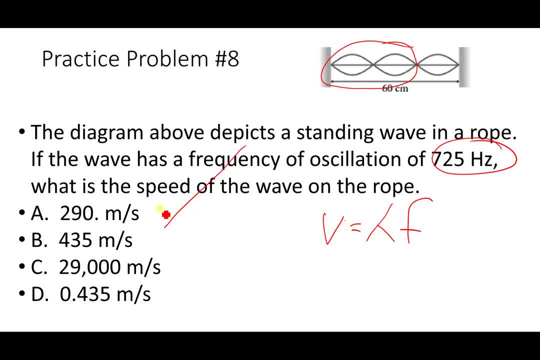 40 centimeters, But notice that all our speeds over here are in meters per second. So 40 centimeters is equal to two-thirds of the string length, 60. So that was 40 centimeters. So our centimeters is 0.40 meters times our frequency of 725 hertz. We multiply that out and we end up. 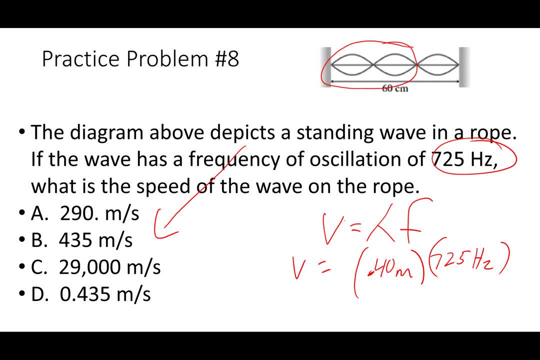 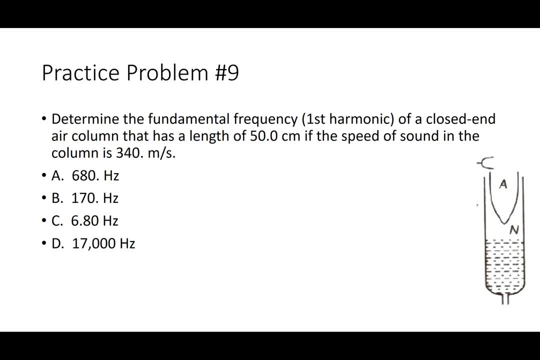 with 290, and our units are going to be meters per second in this case. So 290 meters per second. All right, practice. problem number nine: We have a standing wave in a closed-end air column and we're trying to find the fundamental frequency. 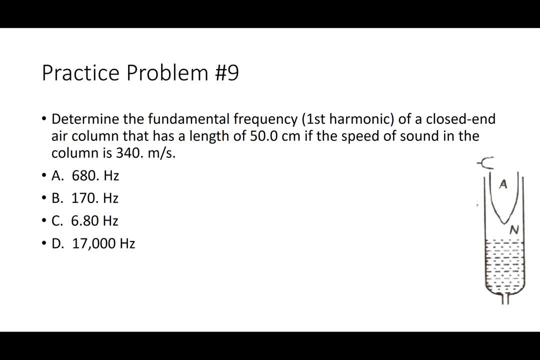 The first harmonic. if we know the length of the air column- 50 centimeters- and we know the speed of sound in that air column is 340 meters per second, Well, again we've got to use the wave equation. Speed equals wavelength times frequency. We're trying to find frequency, so we solve for. 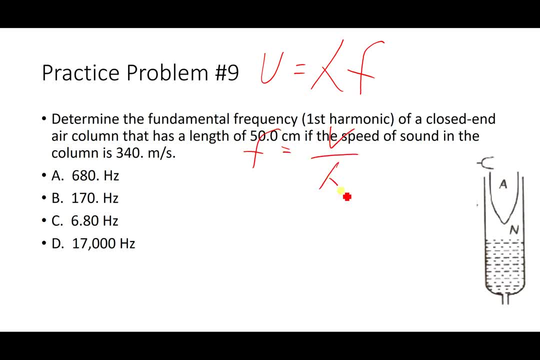 frequency. Frequency is going to equal speed divided by wavelength. We know the speed is 340 meters per second, but we've got to find that wavelength. What we're looking at in this picture is like one-half of one loop and we know that that length is 50 centimeters. We know that. 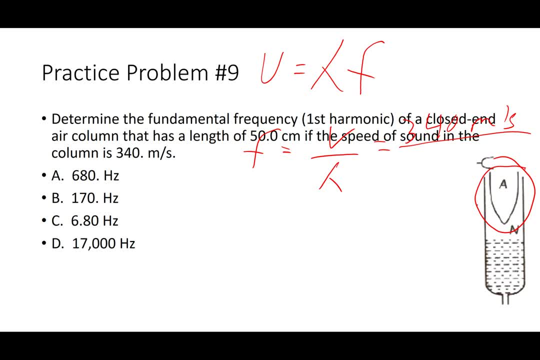 one wavelength is made of two complete loops, So essentially this is one-half of a loop, so four of those, which means our wavelength is four times this air column length. So our wavelength is 200 centimeters. So we need to do this in meters per second. So 200 centimeters is two meters. 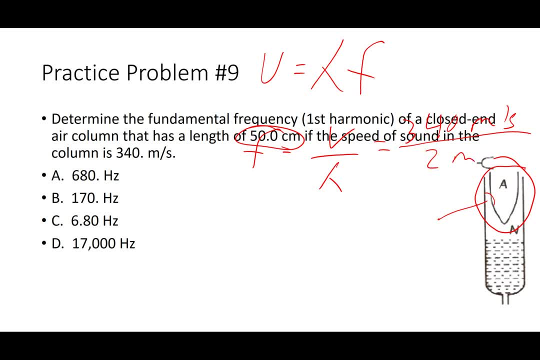 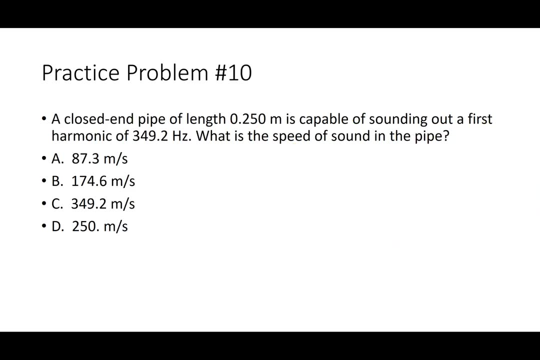 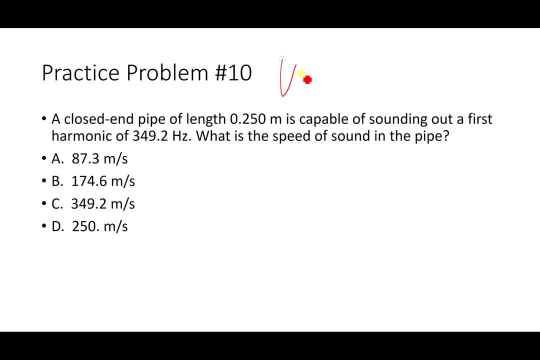 first harmonic at 349.2 hertz. We get a first harmonic at 349.2 hertz. We want to know the speed of sound in the pipe. Again, we have to use the wave equation. Speed is wavelength times frequency. We know the frequency That goes here. Remember that a first harmonic is going to be the 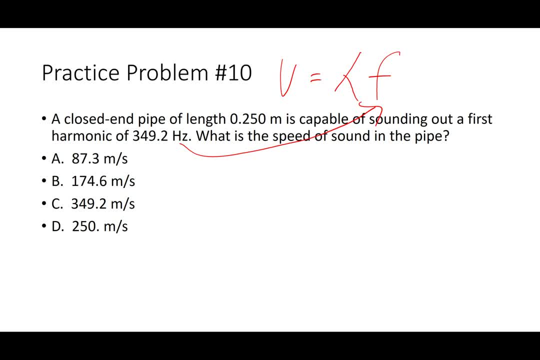 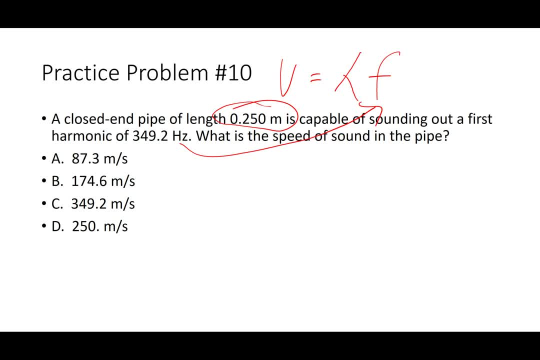 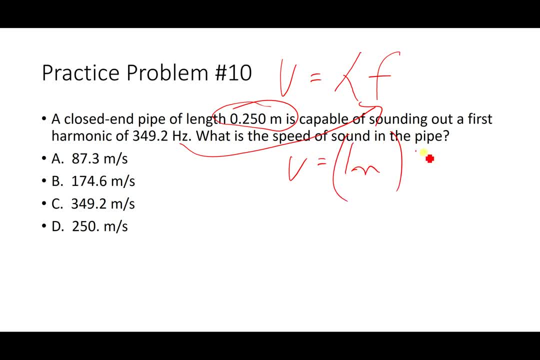 equal to one meter of wavelength times our frequency of 349.2 meters per second. So we're going to end up with a speed of 349.2 meters per second. Again, remember the first harmonic is a fourth of a loop. So to find that wavelength we need to multiply 0.250 times four. So we're 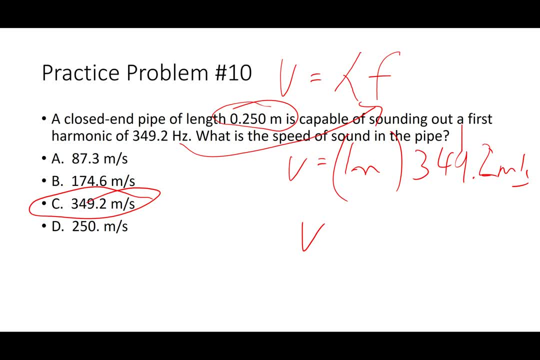 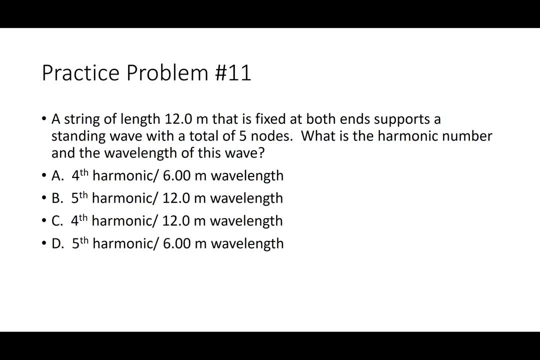 going to end up with a speed of 349.2 hertz. We need to multiply that 0.250 times four to get the wavelength of the actual wave. All right, so practice problem 11.. We have a string of length, 12 meters, fixed at both ends, and we get a standing wave with five nodes. And we want to know the. 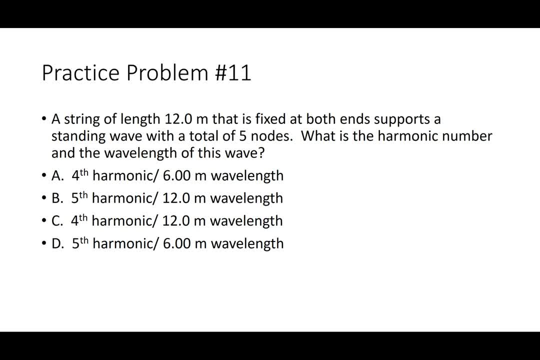 harmonic number and the wavelength of the wave. First of all, remember, the harmonic number is equal to the number of anti-nodes, or you can also find it by taking the number of nodes minus one. So we have four, five nodes minus one, we have the fourth harmonic. this is the fourth harmonic. 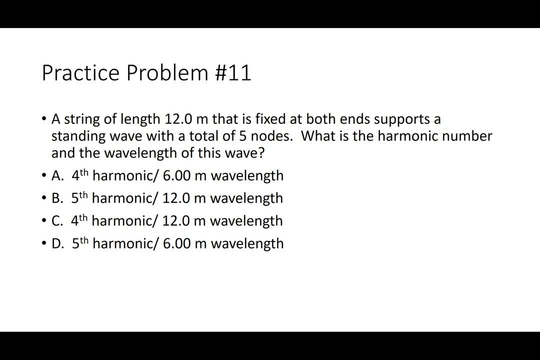 if the wave has five nodes, it's going to have four anti-nodes. if it has four anti-nodes, that means it's consistent, consisting of four complete loops. well, remember that one wavelength is two loops. so essentially, on this string, we have two complete wavelengths. well, the string is 12 meters. 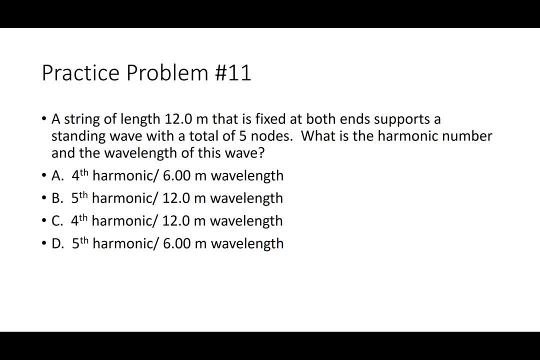 long. we complete two wavelengths in that string, which means the wavelength in this case is half the length of the string. so we're dealing with the fourth harmonic and the wavelength of our wave six meters, half the length of the string. answer a looks good for practice. problem 11: 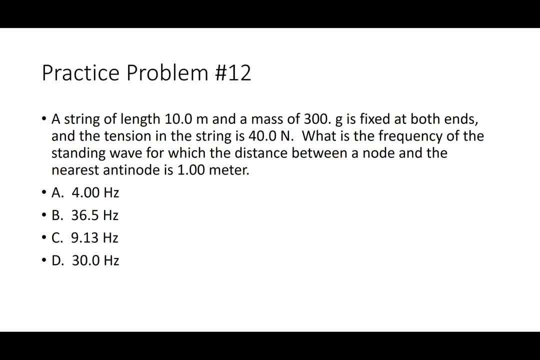 all right, so practice problem 12: we have a string of length 10 meters and mass of 300 grams. it's fixed at both ends, it has a tension in the string of 440 newtons and we want to find the frequency of the standing wave for which the distance between a node and the 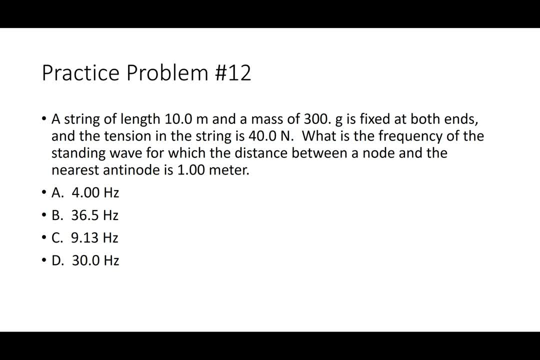 nearest anti-node is one meter. first thing that we've got to do here is find the speed of the wave, and to do that we're going to use this equation: the speed is going to be equal to the square root of the tension force divided by the mass of the string, divided by the length of the. 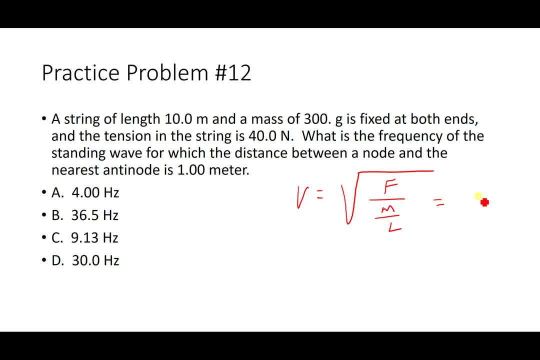 string. so in this case we have the tension, 40 newtons- we have the mass- let's put that mass in kilograms, so point three kilograms- and we also have the length of the string: 10 meters. we have to take the square root of that whole quantity and when 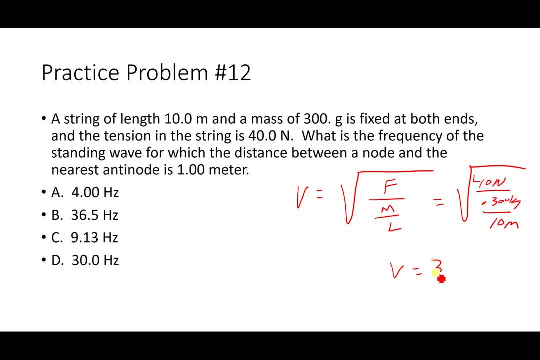 we do, we end up with a speed of 36.5 meters per second. next, we can use the. the wave equation V equals wavelength times frequency. we're trying to solve for frequency, so frequency equals speed divided by lambda. well, we know the speed: 36.5 meters per second. 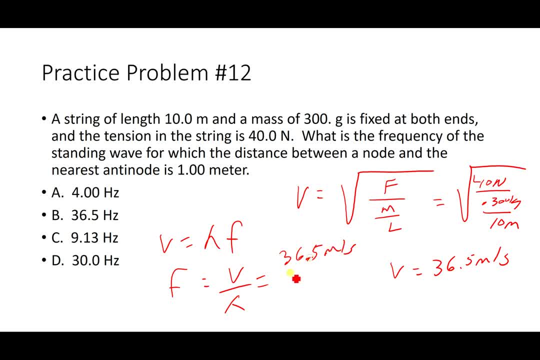 all right, we can get the wavelength from the stem of our question. it tells us that the distance between a node and the nearest anti-node is one meter. well, the distance from a node to an anti-node is essentially half of a loop. remember that a standing wave is made of two complete loops. so this distance from one node. 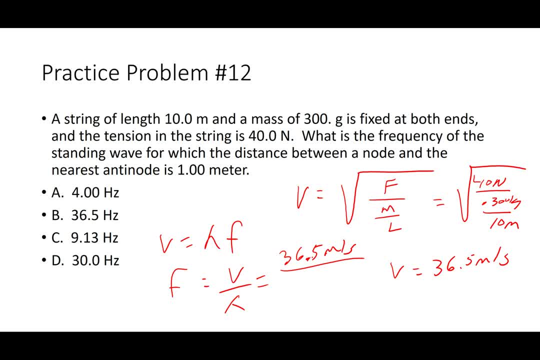 to an anti-node is essentially one-fourth of one wavelength. so if one-fourth of one wavelength is one meter, then a whole wavelength is going to be four meters. our wavelength is four meters, so we take 36.5, we divide it by four meters and we end up with a frequency of 9.13 hertz. 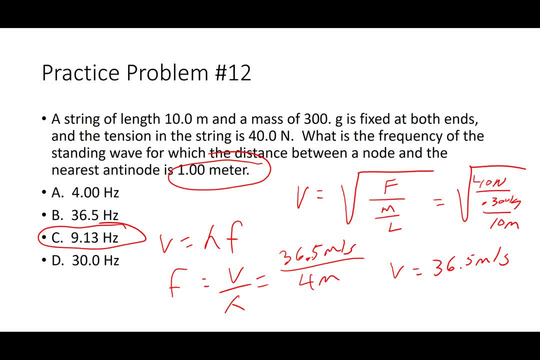 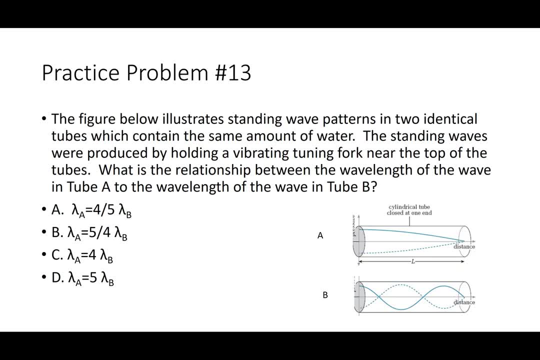 so our answer on practice problem 12 is c. all right, so practice problem 13: uh, the figure below illustrates standing wave patterns in two identical tubes which contain the same amount of water. the standing waves were produced by holding a vibrating tuning fork near the top of the tubes. what's the relationship between the wavelength of? 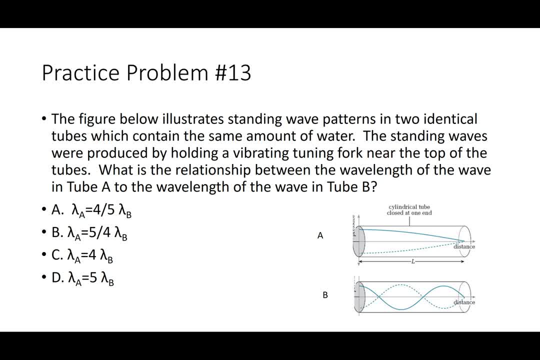 the wave in tube a and the wavelength of the wave in tube b. well notice, in tube a our standing wave is essentially just one-fourth or one-half rather, of one loop, which means we're looking here at really one-half of one loop, which means we're looking here at really one-half of one loop. 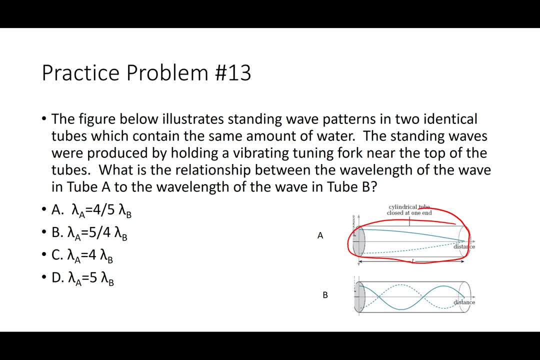 at one-fourth of one wavelength, which means the wavelength of this wave is essentially four times the length of the tube- we'll say four times l- whereas down here the wavelength is much shorter. here we can see one complete wave right there plus one-fourth of another wave. 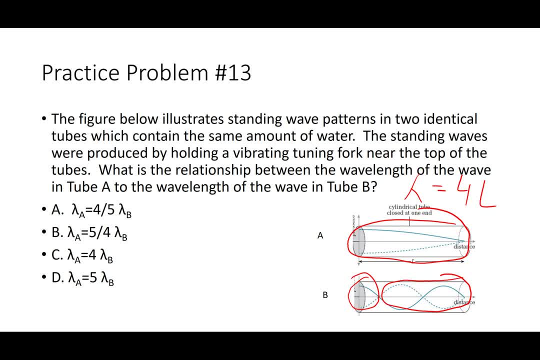 so that means in this string length or in this tube length? rather, we have four-fifths of one wavelength, which means we're looking here at one-fourth of one wavelength. so that means in this string length or in this tube length: another오� Wes forb� bere one and the two, that this means our wave length, this. 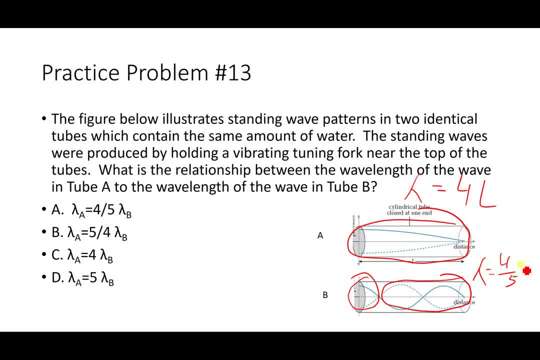 is essentially four-fifths of the length of the tube. So if we compare these, So if we compare these two, what that tells us is that this wave is essentially five times the length of this. so let's look an answer here. looks like our answer here is gonna be wrestling woodee. 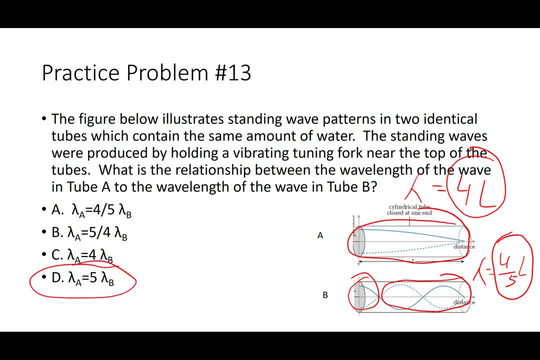 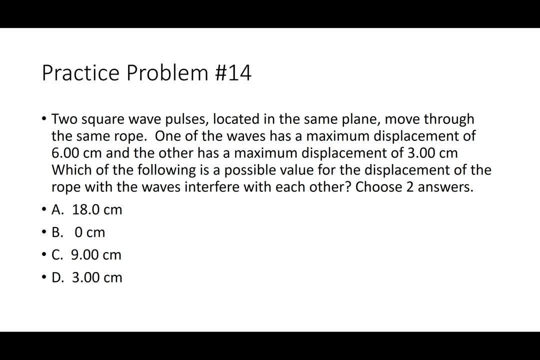 d, wave a is essentially five times longer than wave b. all right practice. problem 14: two square wave pulses located in the same plane move through the same rope. one of the waves has a maximum displacement of six and the other has a maximum displacement of three centimeters. which of the 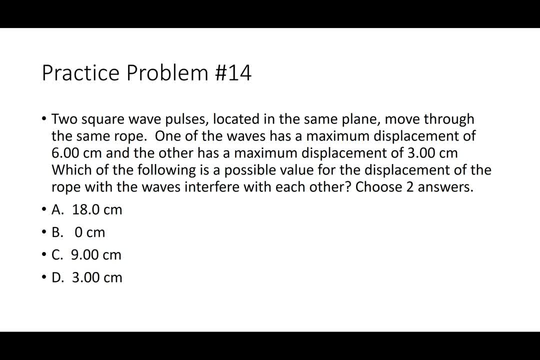 following is a possible value for the displacement of the rope when the waves interfere with each other. choose two answers. all right, when the two waves, when two waves, interfere, their, their summed displacement has to equal the algebraic sum of the individual displacements. so if they're 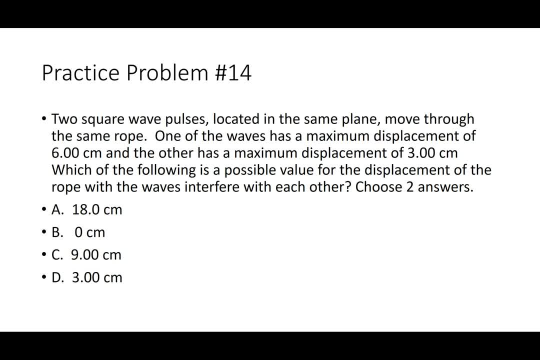 constructively interfering. if they meet crest to crest or trough to trough, we're going to get six plus three, we're going to get nine centimeters. so answer c is a valid answer, you, but we could get it where where a crest of one of the waves meets a trough of the other. so we 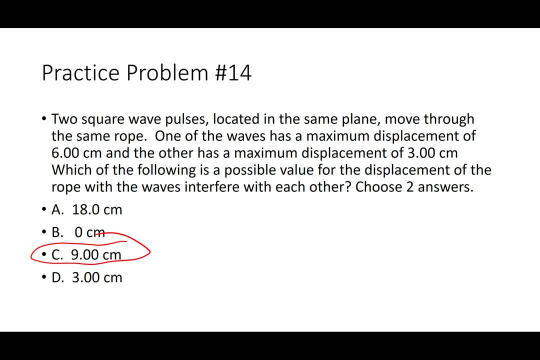 could get a six on top and a three on bottom, or vice versa. that's like adding positive six and negative three, or negative three and positive six. either way, we're going to end up with an answer of three. so if we get positive interference, we're going to get nine centimeters negative interference. 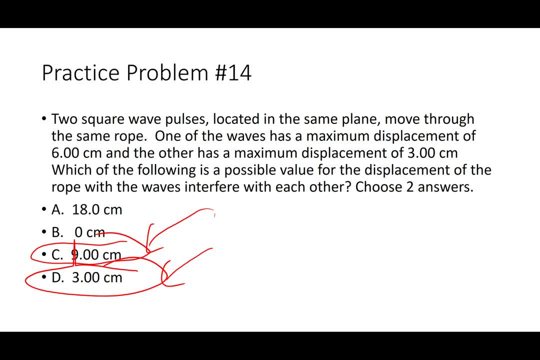 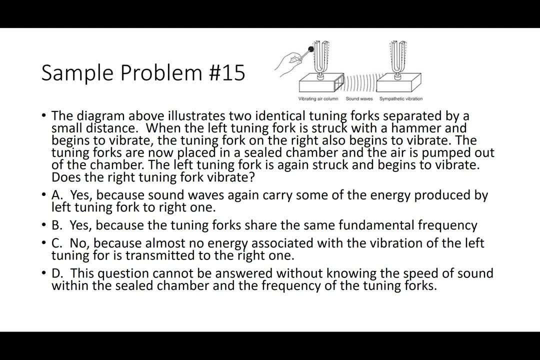 is going to give us three centimeters. so on practice problem fourteen. we're looking at answer c and d. all right, so now we're on practice problem fifteen. the diagram above illustrates two identical tuning forks, separated by small distance. when the left tuning fork is struck with a hammer and begins to vibrate, the tuning fork on the right also begins. 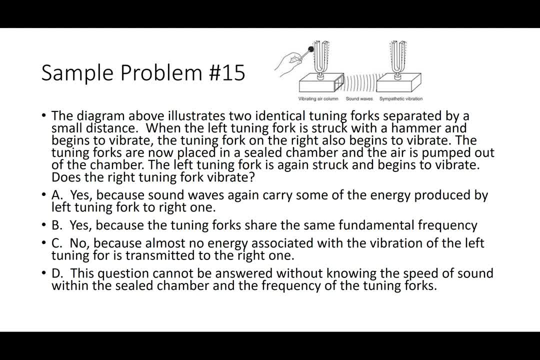 to vibrate, so the sound waves travel. they have similar frequencies, resonant frequencies, so there's some force vibrations. The tuning forks are now placed in a sealed chamber and the air is pumped out of the chamber. The left tuning fork is again struck and begins to vibrate. Does the right tuning fork vibrate? 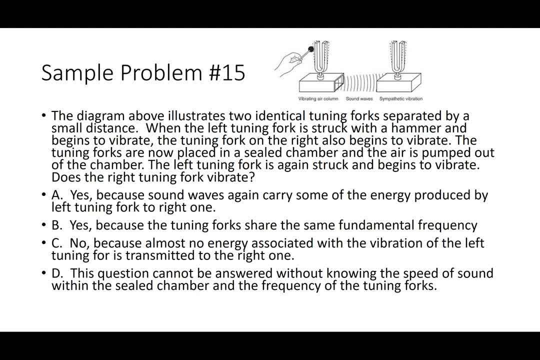 Important thing to remember here is that sound waves, unlike light waves, require medium. They require air. So when we put them in a vacuum chamber that pumps out the air, there's no air, there's no medium and therefore the sound waves 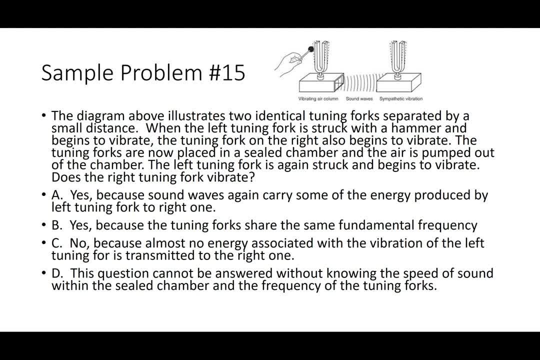 can't move from the left tuning fork to the right one. So the answer we're looking for on this one is C? no, because almost none of the energy from here actually makes it over here and therefore it cannot force that tuning fork to vibrate. All right, practice, problem 16.. The figure below illustrates: 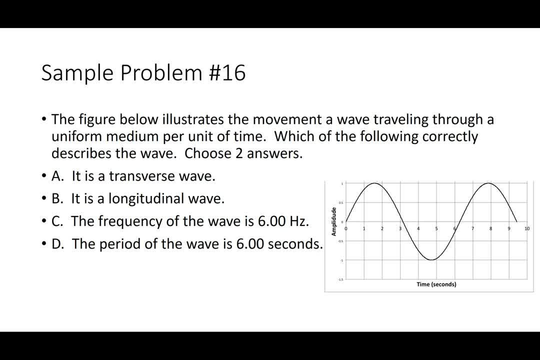 the movement of the tuning fork, The movement of a wave traveling through a uniform medium per unit of time. Which of the following correctly describes the wave? Choose two answers. All right, so we're looking at the amplitude of the wave against time And we 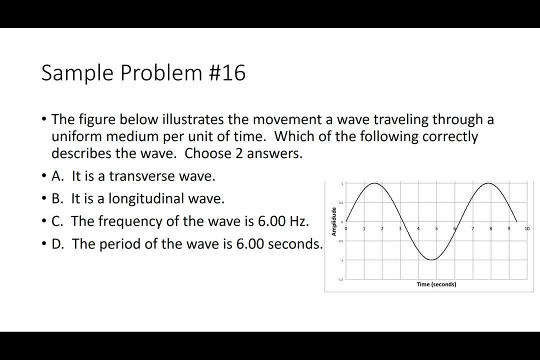 see that the amplitude is vibrating up and down and the wave is moving this way. So that tells us, because the vibrations are in the opposite direction of the movement of the energy. it's a transverse wave, So A looks good. It's not a longitudinal wave. We need to know if either the frequency or the 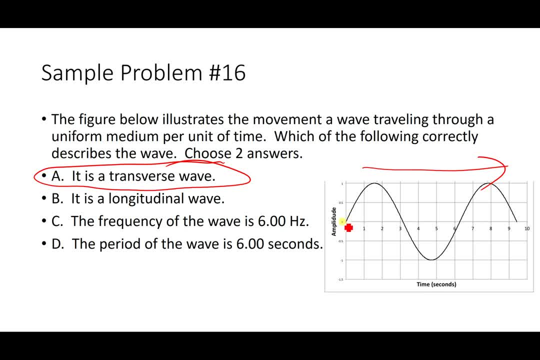 period is six seconds. Well, if we start here, notice this wave goes up, it goes down, comes back up and right here it begins to repeat itself again. So this is one cycle. It takes six seconds for one cycle to occur. That tells me that the 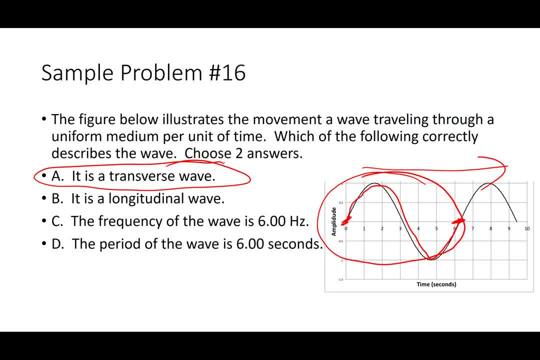 period of this wave is six seconds, The frequency would be equal to one over six seconds. So on practice problem number 16, we're looking at answers A and D, All right, so on to practice problem 17.. We have a student who 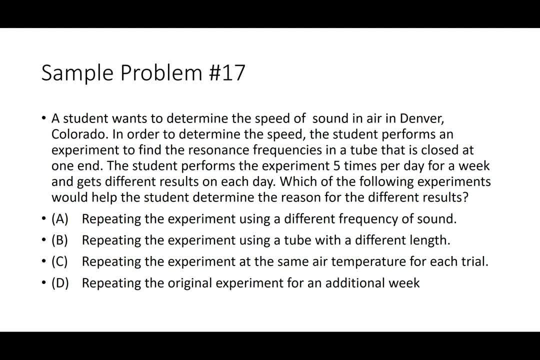 wants to determine the speed of sound and air in Denver, Colorado. In order to determine the speed, the student performs an experiment to find the resonant frequencies in a tube that is closed at one end. So much like the problems we worked earlier. The student performs the experiment five times per day for a week. 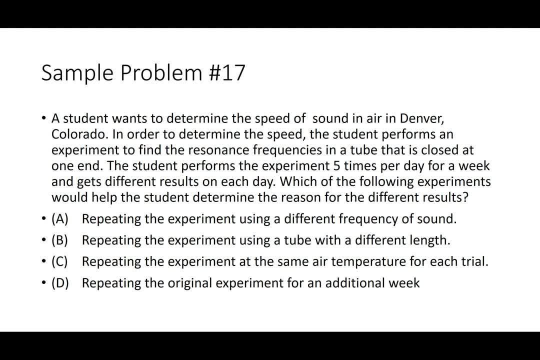 and gets different results on each day. Which of the following experiments would help the student determine the reason for the different results? Okay, A, using a different frequency. B- using a tube of a different length. C looks like the correct answer here, Because what you've got to remember is that the speed 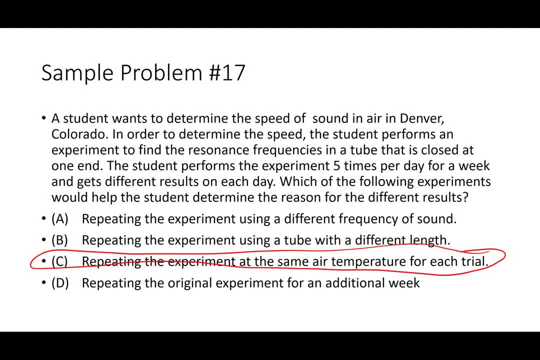 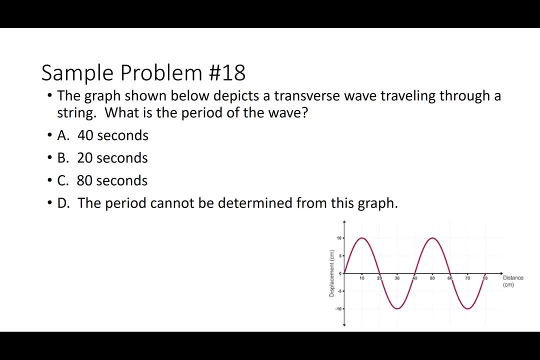 of sound varies with temperature. As the temperature of the air increases, the speed increases. So we're looking at C as the best answer here On practice problem 17.. All right, practice problem 18.. The graph shown below depicts a transverse wave traveling through a stream. What's the period of? 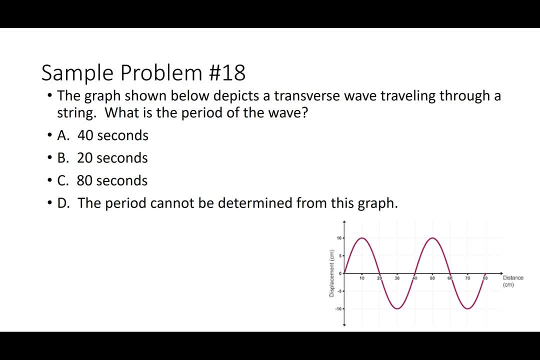 the wave. Some of you are going to not pay attention to the graph and you're going to say, okay, the wave goes up and down and back up and it starts over here, So the period is 40.. Well, you'd be incorrect if you did that, because this: 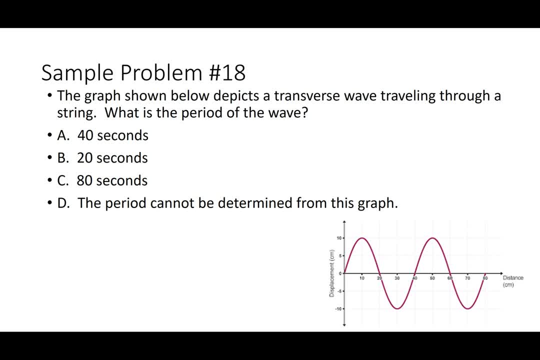 is not a displacement against time graph. This is a displacement against distance graph. So what this is saying is that as the wave displaces this far and a point displaces this far, the wave actually moves this far down the stream. This particular graph does not give us the information we need to determine the 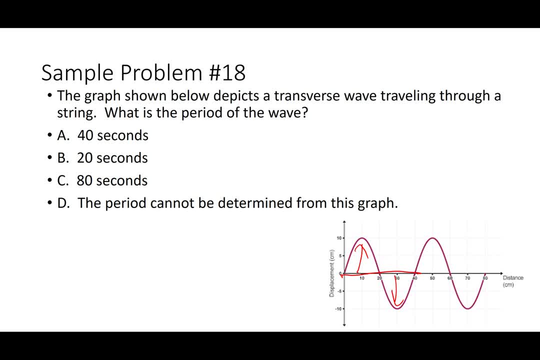 period or the frequency. This particular graph, a displacement versus distance graph, would allow us to determine the wavelength. It will not allow us to determine the period or the frequency. So our answer here is B. All right, so we're back to number 19.. It looks like the same problem, but 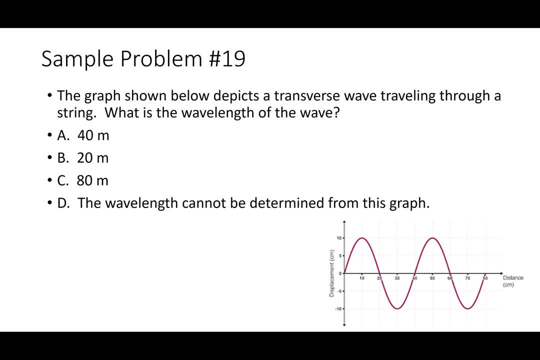 this time the problem is asking us to find the wavelength, not the period. So again we see that the wave starts here, it goes up, it comes back down and then, right here, it begins again. So here we're looking at one complete cycle, one. 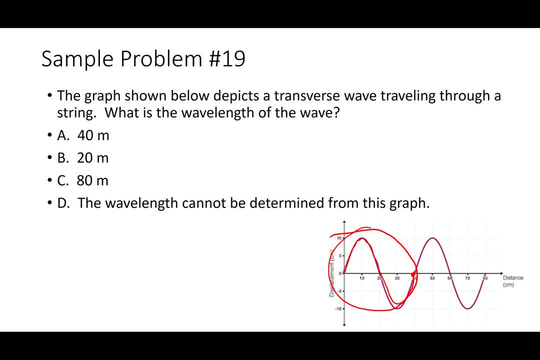 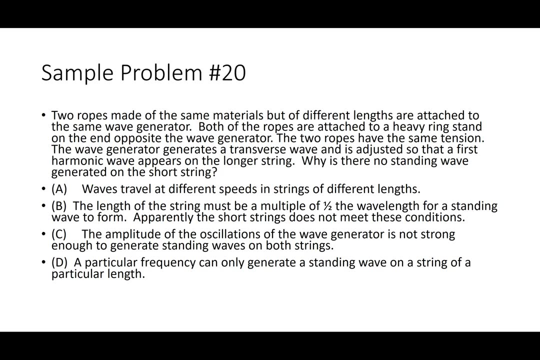 complete wave, one complete wavelength, and that wavelength is 40 centimeters long. so this is 40 ight meters. this should say 40 centimeters. let's get that correct. so answer here is answer a. all right, so this time we have two ropes made of the same materials but of different lengths. 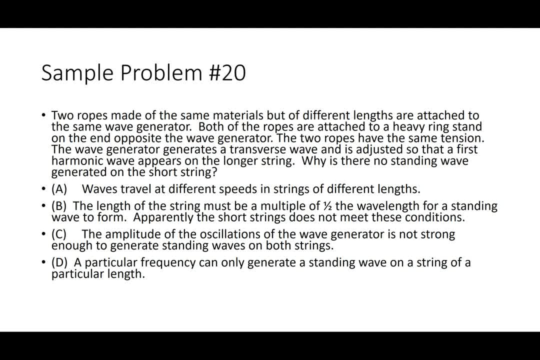 and they're attached to the same wave generator. both of the ropes are attached to a heavy ring, stand on the end opposite the wave generator. the two ropes have the same tension. the wave generator generates a transverse wave and is adjusted so that a first harmonic wave appears. 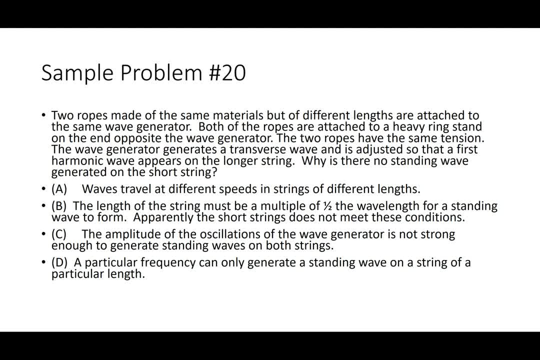 on the longer string. why is there no standing wave generated on the shorter string? well, if we look through our answers here, the best answer is b- the length of the string must be a multiple of one half the wavelength for a standing wave to form, and the shorter string just doesn't meet those conditions. so again, standing waves. 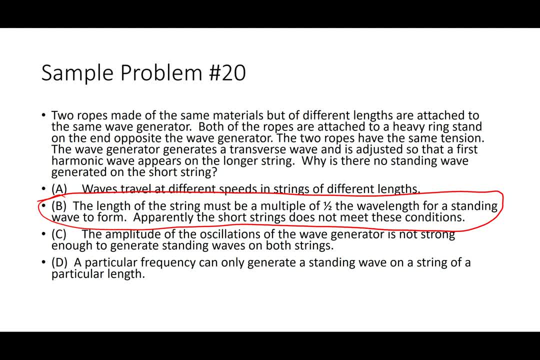 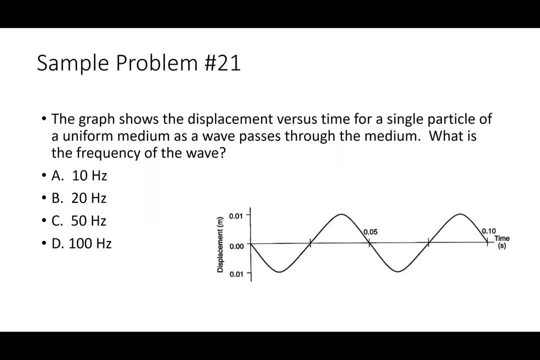 can only form on strings that have links that are multiples of half the wavelength of the wave generator. so we're going to look at the first problem, all right, so press problem 21. the graph shows the displacement versus time for a single particle of a uniform medium. as a wave passes through the medium, what's the frequency of the wave? so we're 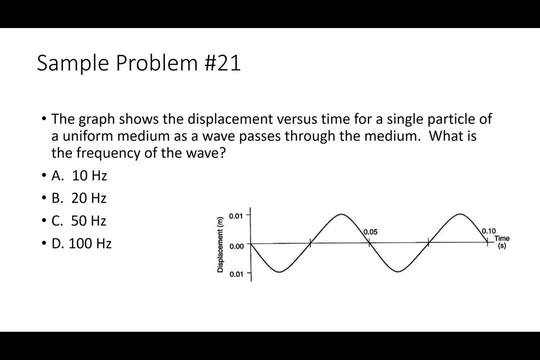 looking at a displacement against time graph. that tells us that from this graph we can find frequency, we can find period. if we start at this point, the wave goes down, it goes up, it comes back and then right here that wave begins to start over. so this portion is one complete wavelength. 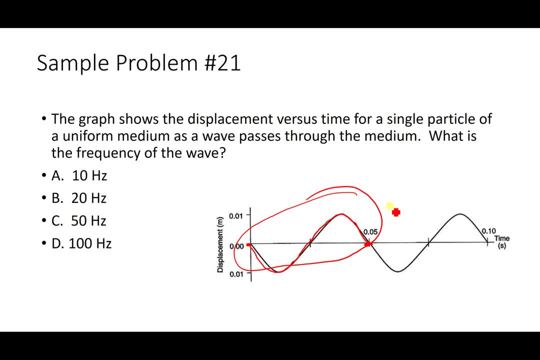 and for that to happen it took 0.05 seconds. well, that means that the period is 0.05 seconds. we're looking in this case for the frequency. we know that frequency is one over the period, so one over 0.05 seconds, and when we do the math on that, we end up with a frequency of 20. 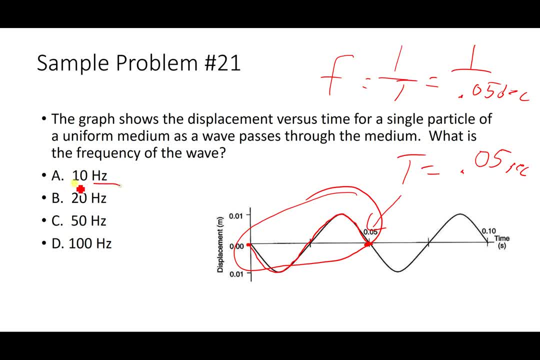 hertz, 20 cycles per second, 20 waves per second. answer b looks good for practice. problem number 21: all right, so same graph we used on the last problem. remember this is a graph of for a single particle in a medium and all the particles doing is vibrating up and down. 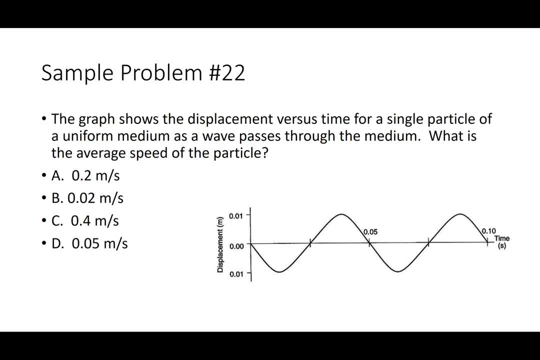 we're trying to find the, the speed of that particle. so it vibrates down one point or 0.01 meters, and then it vibrates back up 0.01 meters, and it does that in 0.05 seconds. so if we're trying to find the speed, this thing travels. 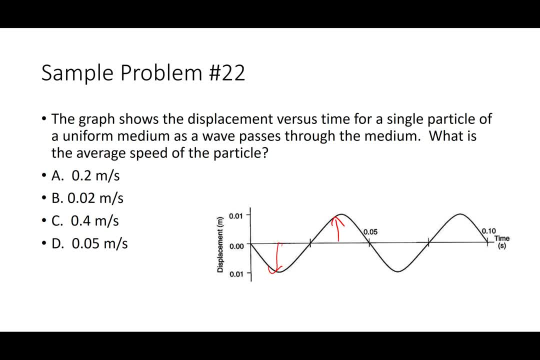 0.01 plus 0.01, so it travels 0.02 meters and it does that every 0.05 seconds. we know speed is essentially distance divided by time. so if we go 0.02 divided by 0.05, we end up with answer c: 0.4. 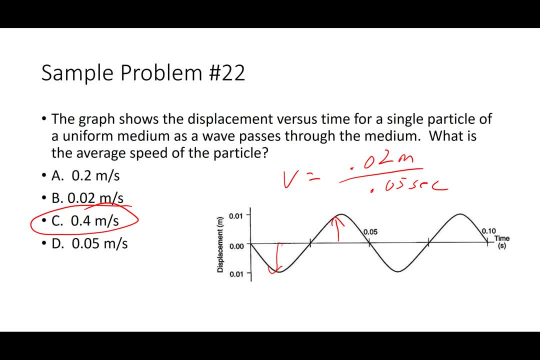 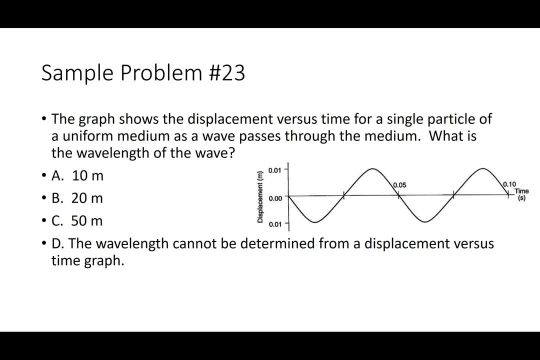 meters per second is our speed of this particle. all right, so practice. problem 23: same graph we looked at earlier, remember this is a graph for a single point, single particle in a medium, as the wave passes through the medium and we're trying to find the wavelength of the wave. 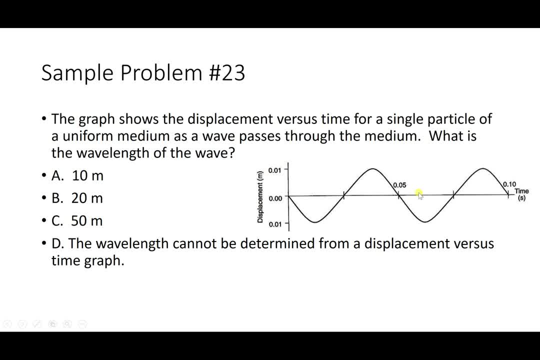 now note: this is a displacement versus time graph. if we're going to find the wavelength, we need a displacement versus distance graph- a distance the wave traveled. we don't have that here. that's telling me that this graph will not allow us to determine the wavelength. so our answer on 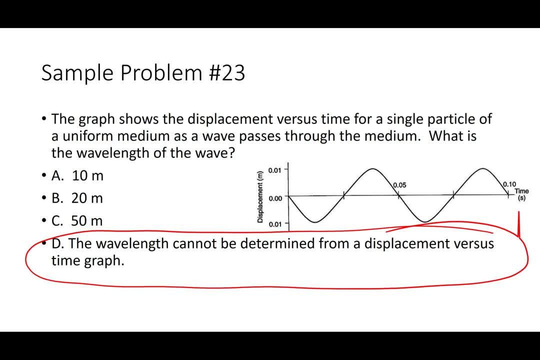 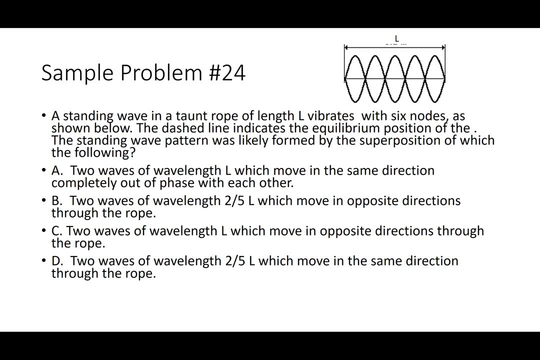 this particular question is d. if we want to find the wavelength from a graph, we need to have a displacement versus distance graph. all right, so number 24, a standing wave and a taunt rope of linked l vibrates with six nodes. and notice, if it has six anti or six nodes, it's going to have five. 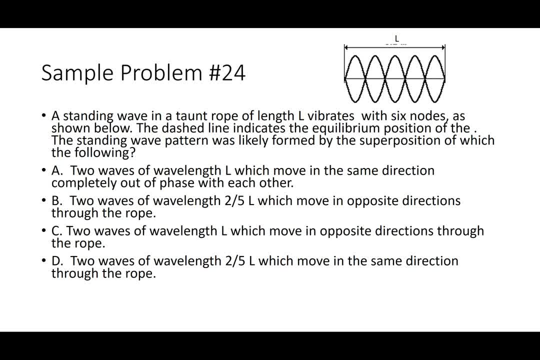 antinodes line indicates the equilibrium position of the wave. The standing wave pattern was likely formed by the superposition of the following: Remember: superposition essentially means they're placed on top of each other where they will interfere. So remember that standing. 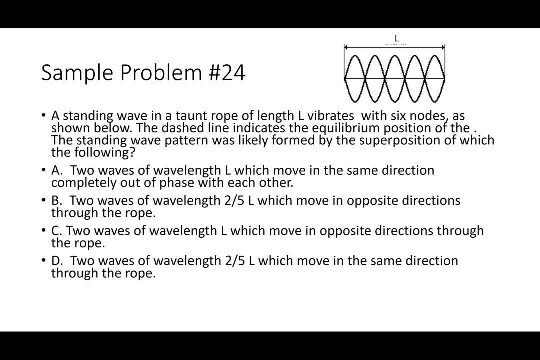 waves in a string occur. when a wave moves through the string, vibrates, bounces back and then meets the next wave. Those waves are going in opposite directions. So first of all, any wave on here that says the same direction we can probably eliminate that. 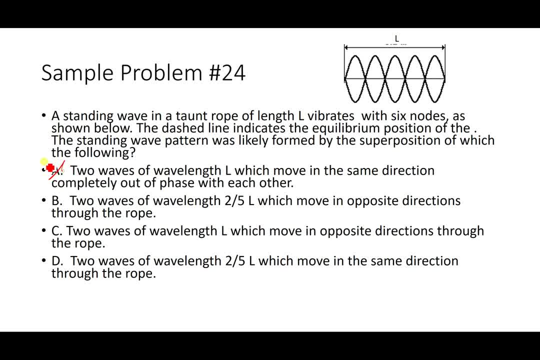 choice. So that would eliminate A and it would also eliminate D. Our two waves need to be moving in opposite directions. So the other thing that we need to look at is the wavelength. Remember that one wave is making a wave. So if we look at the wavelength of the wave, we need to look at the wavelength. 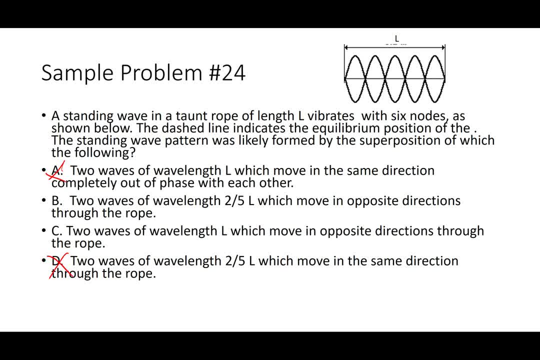 of the wave. So if we look at the wavelength of the wave, we need to look at the wavelength of two complete loops. So if we look at the length of the string, there's one wave here, one complete wavelength, another complete wavelength and then a half of a wavelength. 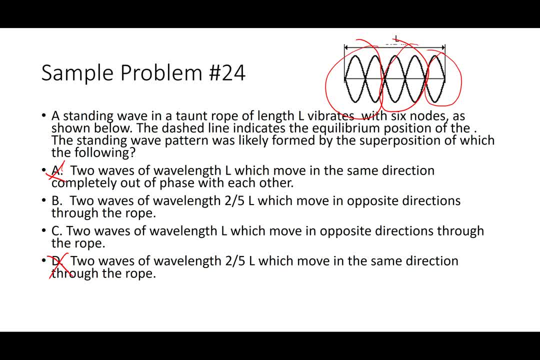 So we're looking on this wave at five halves of a wave, 2.5 waves on that one string, which tells me that the wavelength of the waves that formed this wave were 2 fifths times the length of the string. Only two out of five were one wave. So, knowing that that the wavelength of the 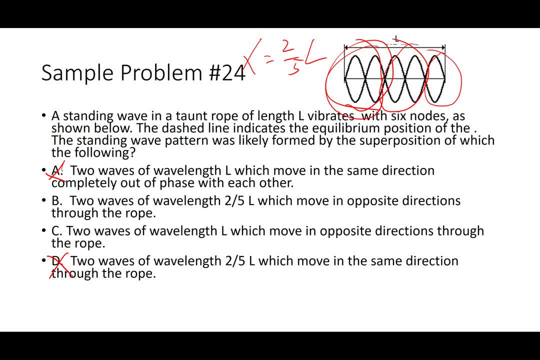 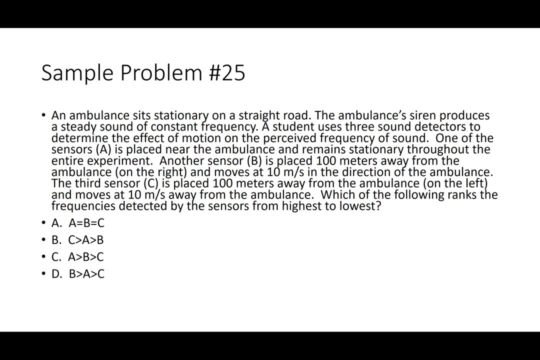 waves that formed this standing wave were 2 fifths times the string length. the answer we're looking for here is B. All right, so the next problem, number 25,. an ambulance sits stationary on a straight road. The ambulance's siren produces a steady sound of constant frequency. A student uses three sound detectors to determine the effect of motion on their 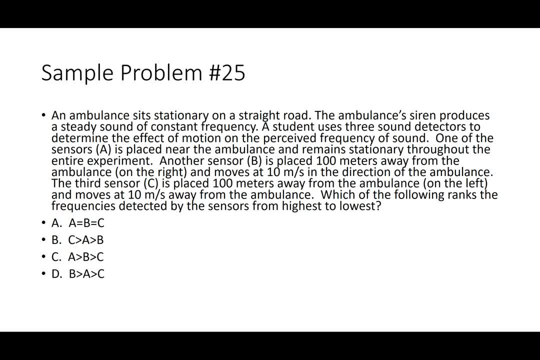 perceived frequency of sound. One of the sensors, A, is placed near the ambulance and remains stationary throughout the entire experiment. Another sensor, B, is placed 100 meters away from the ambulance on the right and moves at 10 meters per second in the direction of the ambulance. The third sensor, C, is placed 100 meters away from the ambulance on the left and moves at 10 meters per second away from the ambulance. Which of the following ranks the frequencies detected by the sensors from highest to lowest? 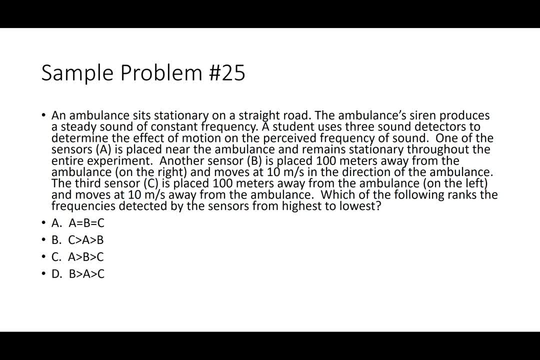 So remember that when a sensor moves toward a sound source, the wave fronts get compressed together And what the sensor picks up is actually waves of a higher frequency than what is actually being released by the source. On the other hand, when a sensor moves away from a sound source, the wave fronts are stretched out, So the sensor picks up a frequency that's actually lower than the real frequency. So what that tells me is that the sensor is 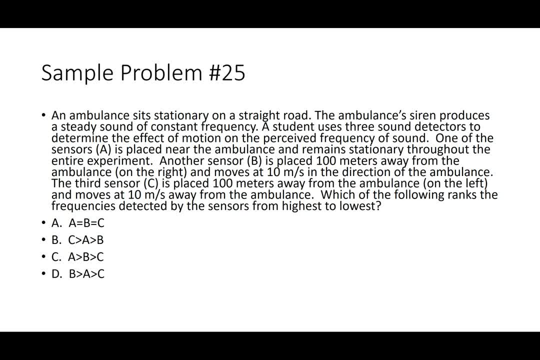 moving toward the sound source is going to have the higher frequency, That's B. So B is going to have the highest frequency. A is just sitting there. A is going to pick up the real frequency of the source. C, on the other hand, is going to have a lower frequency than the source. So this looks like answer D is our correct answer. This is a good example of the Doppler effect: Motion. 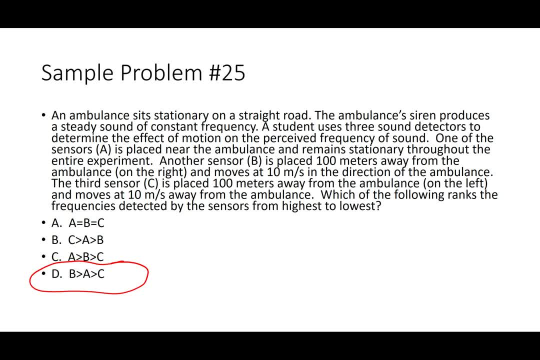 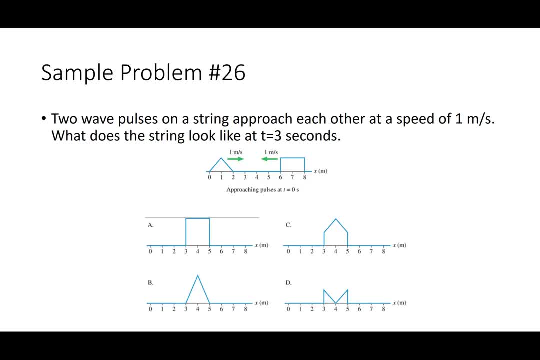 effects the perceived frequency of sounds that are picked up by either a person's ear or, in this case, by a sound sensor. All right, So this is the last practice, problem number 26.. Two wave pulses on a string approach each other at a speed of one meter per second. So notice, they're starting off right. Let's think of the center of the waves. So this one's at one. So after one second the center would be here Two seconds. it would be here Three seconds. it would be right here. 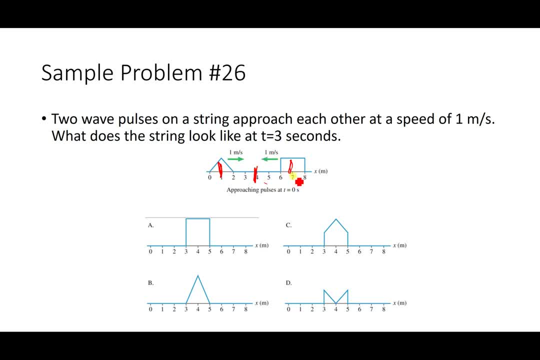 This one's starting at seven. After one second the center would be at six, Two seconds at five, Three seconds at four. So their centers are going to meet at the four meter mark at three seconds. Notice that both of them are pointed up. So their centers are going to meet, They're going to constructively interfere, And remember that the displacement of the combined waves is going to be the algebraic sum of the displacements of the original waves. 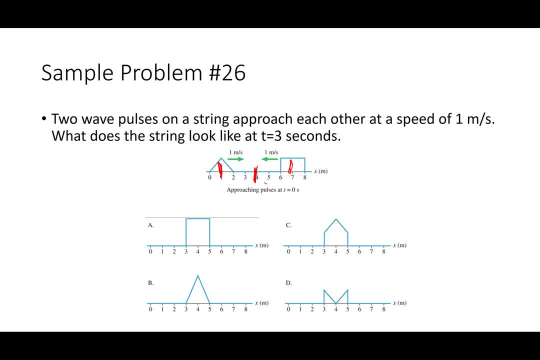 So those are going to add together constructively And what we're going to end up with is something that looks like the two combined. Answer C Forgot about one thing. We have a free response question that we need to look at as well. 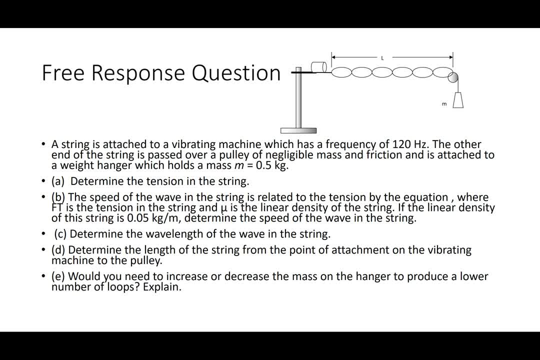 All right. So we have a string attached to a vibrating machine. So this is the vibrating machine over here with a frequency of 120 hertz. The other end of the string is passed over a pulley, So this would be our pulley right here. 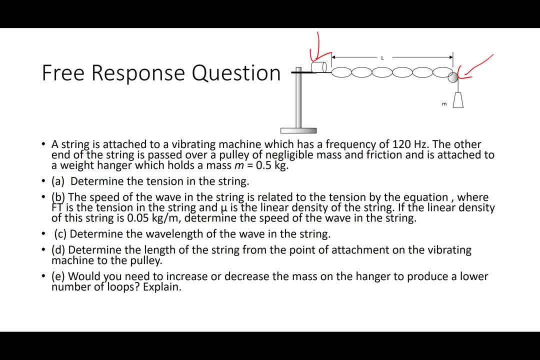 And we're going to say that this pulley is attached to a weight hanger. What is the weight that we're going to see here? And it's attached to a weight hanger which holds a mass of point five kilograms. That would be this Determine the tension in the string. Well, the tension in the string is essentially going to be caused by the weight of this hanging mass, Because it's going to be pulling down And the pulley will translate that to being pulled across. So the tension in the string, in this case, is going to be equal to the weight of this mass. Well, we know that weight equals mg, So weight is going to be equal to the weight of the string. What we would do is we'd just pull it down. 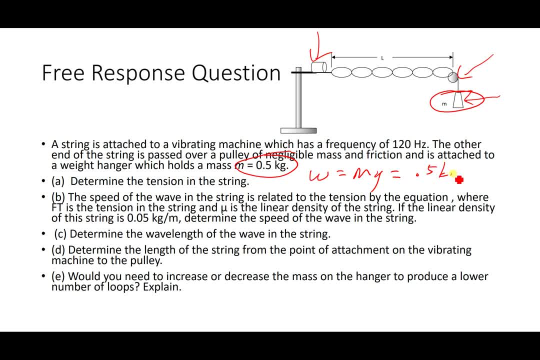 equals 0.5 kilograms times. we'll just use 10 for g. So we're gonna end up with a tension force of five newtons. Second part: the speed of the wave in the string is related to the tension by the equation which we'll talk about in a second. 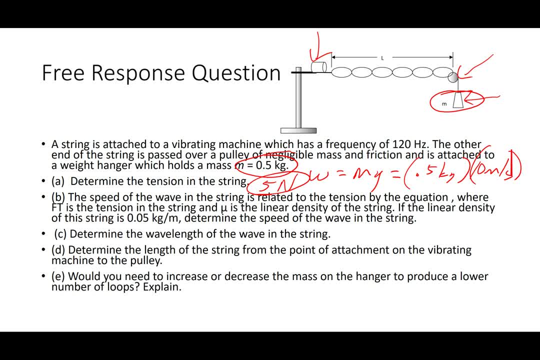 where the tension in the string and where ft is the tension in the string and mu is the linear density of the string. If the linear density of the string is 0.05, determine the speed. So, again, this is the equation we're talking about. 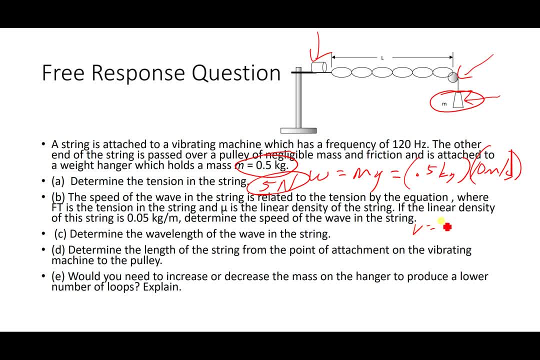 Speed equals the square root of the tension force divided by mu, And remember that mu is essentially the mass over the length of the string. So we're gonna plug in our tension force of five newtons, We're gonna plug in our mu, which is 0.05 kilograms per meter. 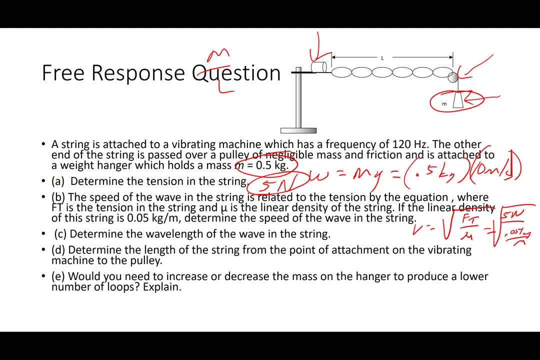 We're gonna divide that and then take the square root of both sides And we're gonna end up with our speed of 100 meters per second. Next, we wanna determine the wavelength of the wave. Well, we'll do that down here at the bottom. 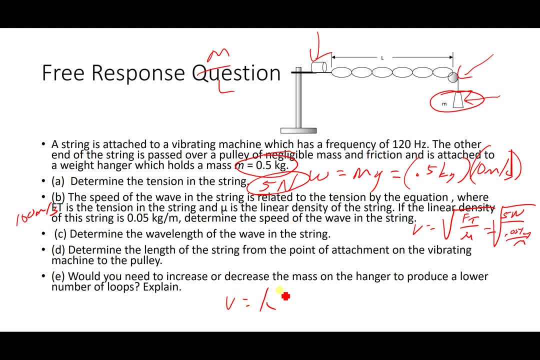 We'll have to use the wave equation. We're trying to find wavelength or lambda. So lambda is gonna be equal to the speed of the wave divided by the frequency of the wave. Well, the speed we just calculated to be 100 meters per second. 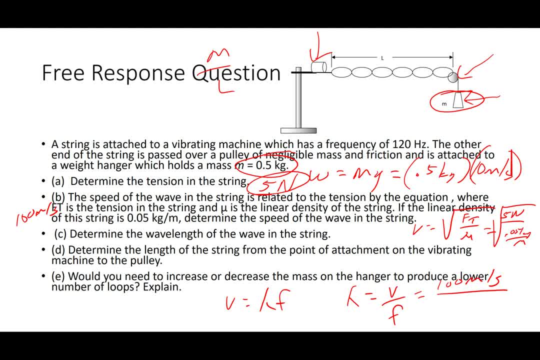 And the frequency is gonna be the frequency of our vibrating machine, which is 120 hertz. So we do the math there: 100 divided by 120.. Our answer on part C is gonna be 0.83 meters. D determine the length of the string. 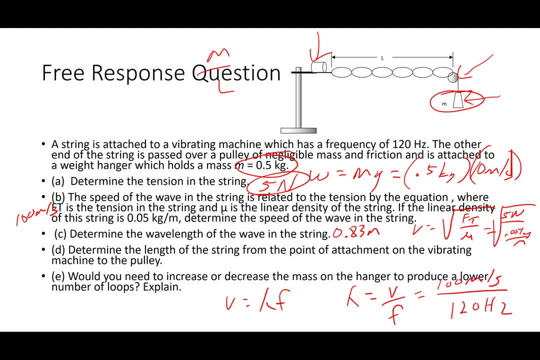 from the point of the attachment on the vibrating machine to the pulley. Well, here's the deal. We know the wavelength of our wave And remember, the wavelength of a standing wave is made up of two loops. So we have one wave, two waves, three waves. 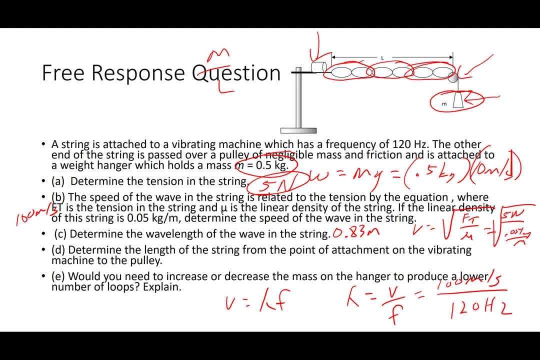 So we have three complete wavelengths on our string. So to find the length of the string we're gonna say three times our wavelength of 0.83 meters. So we're gonna say three times our wavelength of 0.83 meters. So we're gonna say three times our wavelength of 0.83 meters. 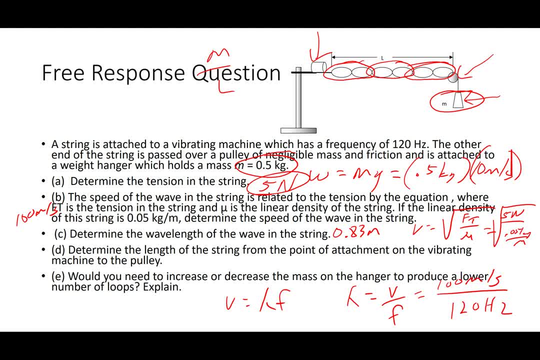 So we're gonna say three times our wavelength of 0.83 meters. Three times 0.83 is gonna give us about 2.5 meters for the length of our string. And then finally, would you need to increase or decrease the mass on the hanger? 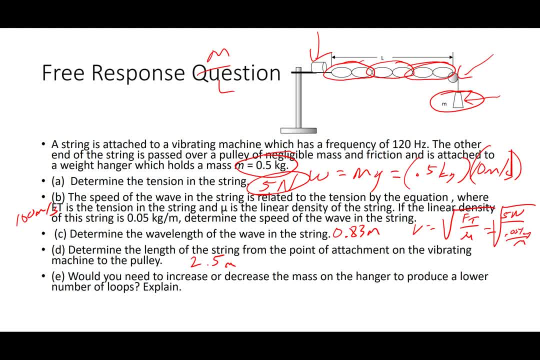 to produce a lower number of loops, All right, so if we had a lower number of loops, that would mean that the wavelength of the wave is longer. We can't change the frequency. The frequency is determined by the vibrating machine. So if the wavelength gets longer, 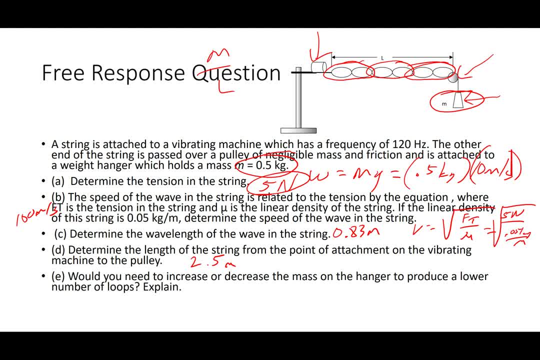 that means the speed of the wave has to increase. Well, the only way we can increase the speed in this particular string is by making it have more tension. To make it have more tension, we're gonna have to increase the mass on the hanger. 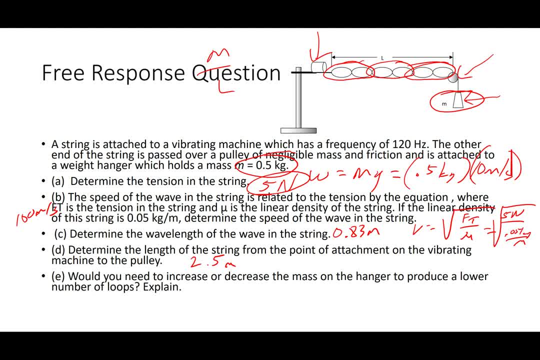 So increasing the mass on the hanger will increase the tension in the rope, which will increase the speed of the wave going through the rope. And since the frequency can't change because it's determined by the vibrating machine, the wavelength will then get longer. 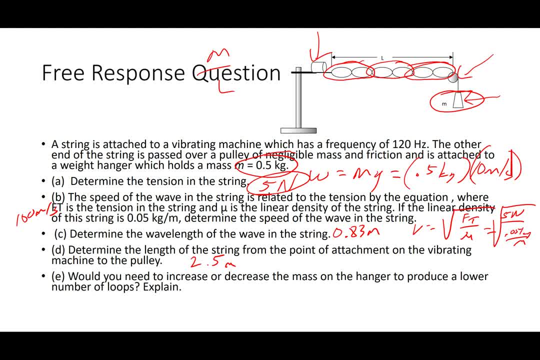 So we're going to need to increase the mass of the mass on the hanger. All right, that's it for our waves practice problems. Hope that helped.